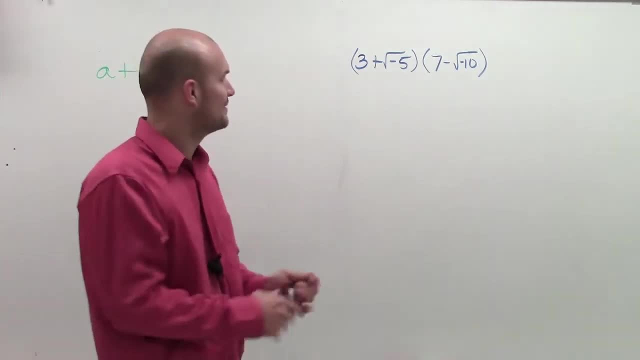 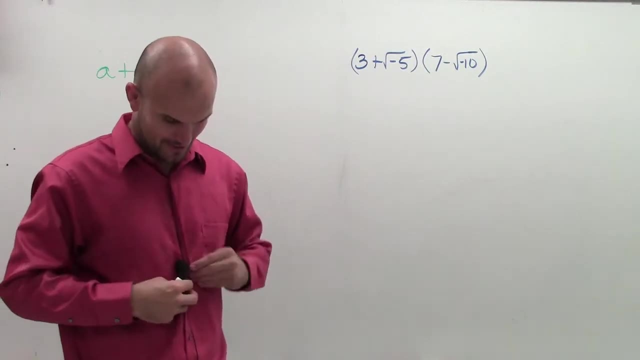 I start to get upset inside and wonder where do my markers go every time? Okay, so what I have here- don't want to cover that up- that's so you guys can hear. Alright, what I have here is I have a binomial and it has some square root of negative numbers, so that 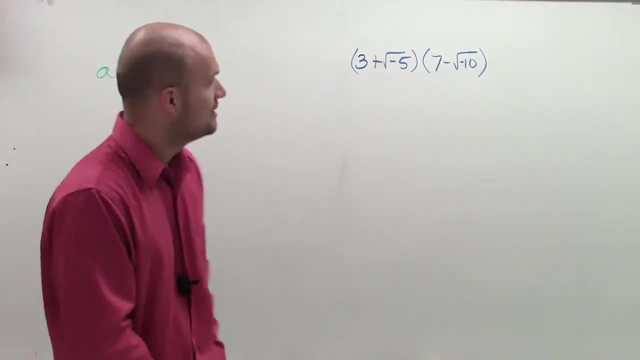 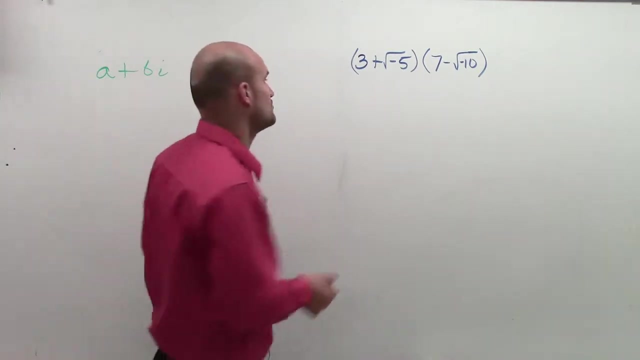 form means I'm going to have to deal with some complex numbers at the end. Now. previously I showed you a problem very similar to this and I used the square method to multiply binomials. You can also use what we call the FOIL method. Remember FOIL represents. 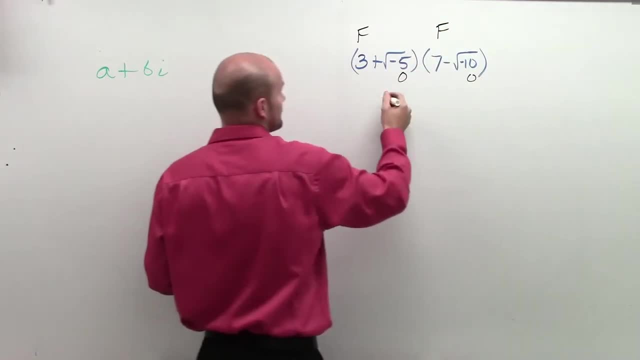 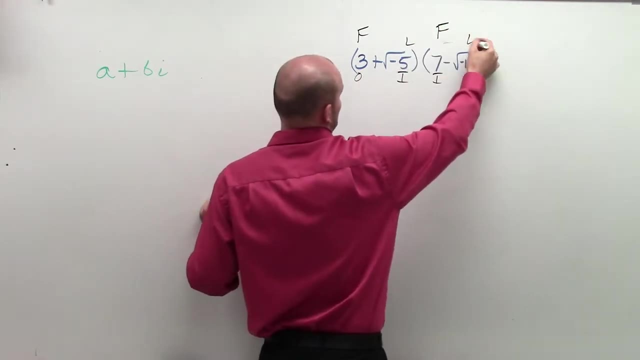 the first. then we talk about our outer terms. that's not your outer. These are your outer, your inner and then the last last terms over here. So what we're going to do is we're going to multiply. When multiplying this out, remember you're doing distributive property. 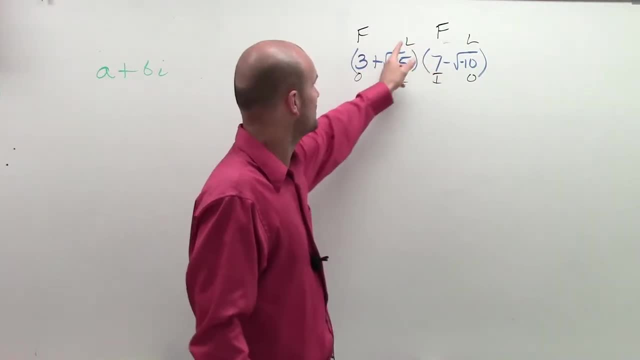 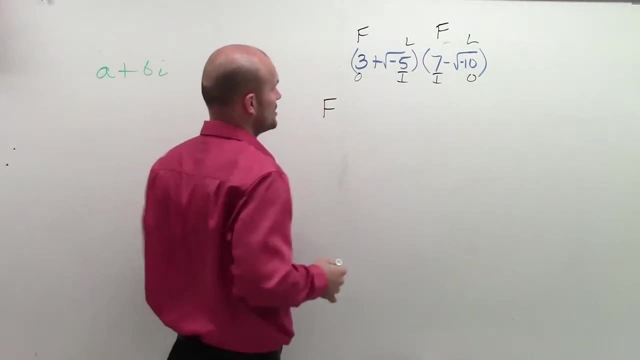 First times, first out, times out Inner times, inner last times last. So really it's just a way to kind of do distributive property easily that we can remember. So let's do our first two terms. We have three times seven. That's pretty good. 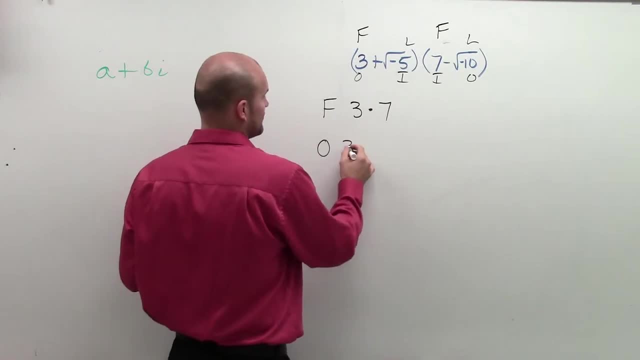 I like that. Outer terms: It's going to be three times negative, square root of negative ten. Inner terms: We have square root of negative five times seven And then we have the last, which is going to be the square root of negative, five times the square root of negative ten. 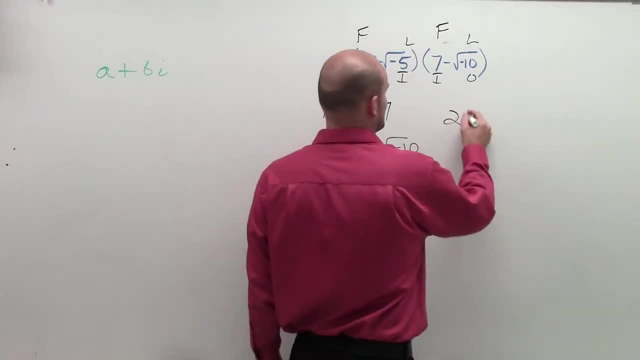 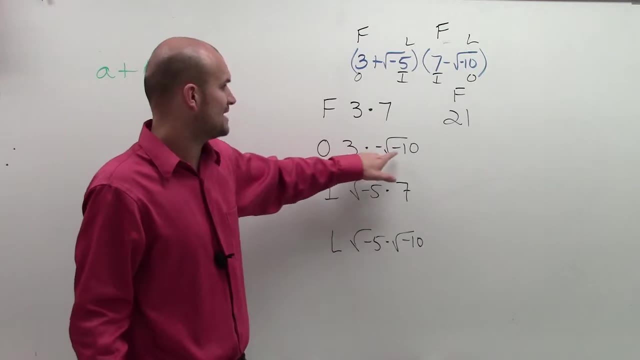 Okay, so first, that's pretty easy. Let's write that right. So that's going to be 21.. I'm actually now going to Do that horizontally so you can see what it looks like. Outer is going to be three times negative. square root of ten is going to be a negative. 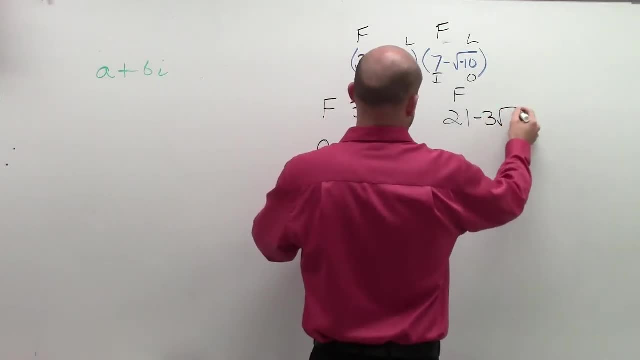 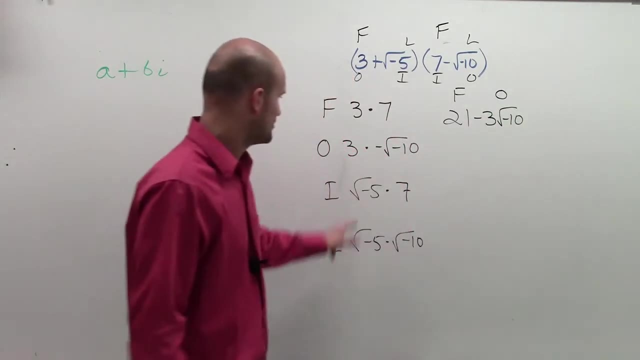 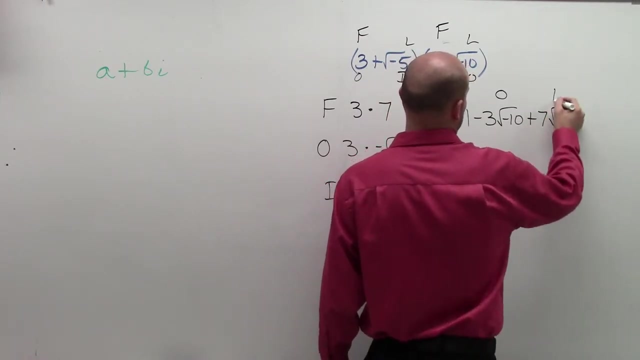 3 square root of negative 10.. Inner is going to be 7 times the square root of negative 5. So that's going to be plus 7 times the square root of negative 5. That's what we call the inner. 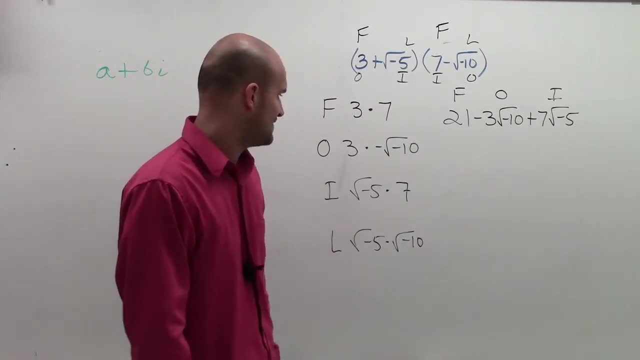 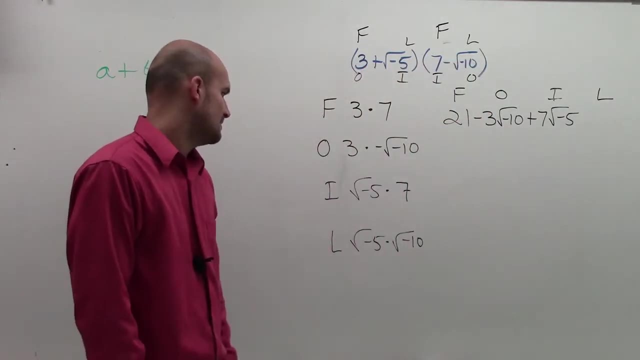 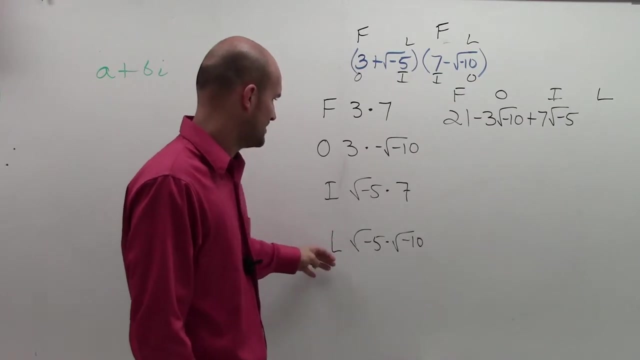 And the last one is: we have last, which would be the square root of negative 5 times the square root of negative 10.. And then which C we could have is going to be: if you remember when we did this, I want to show you that.